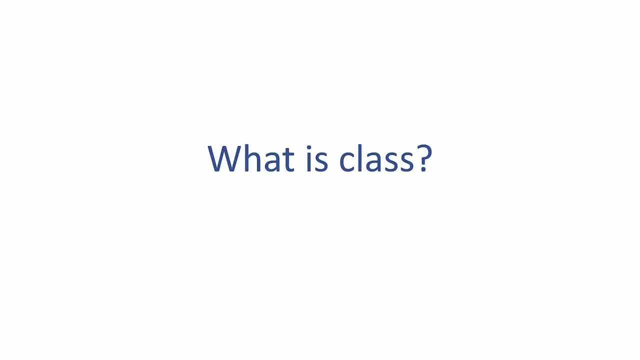 It applies to most of the other programming languages as well, and it falls under a common paradigm called object-oriented programming. Okay, so let's see what is class When you talk about human beings. it has. every human being has a common set of properties. 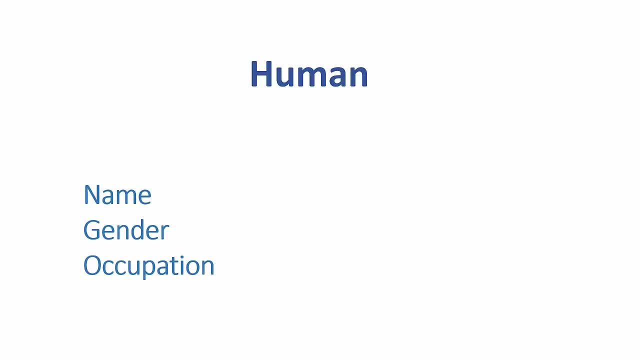 such as name, gender, occupation, etc. Also, every human will be doing some kind of common activities, such as speaking, doing work or sleeping. So the first set of properties that we cover are called properties in object-oriented programming world, And the activities that human performs are called methods in object-oriented programming. 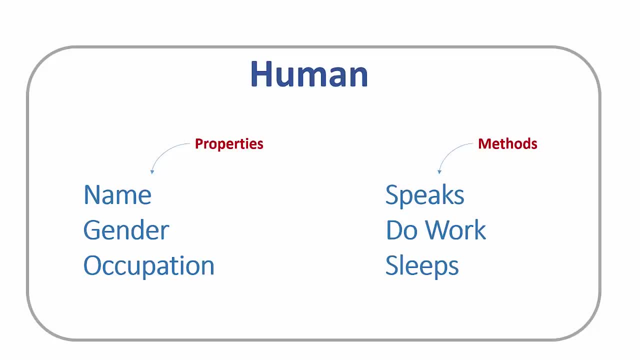 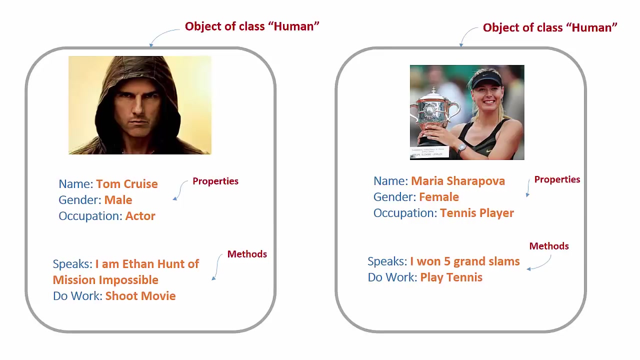 Thus, properties and methods, forms a central entity called a class. So here, human is a class which has two central component, which is properties and methods. so class is nothing but an abstraction of some entity which contains common set of properties and matters. okay, what is object then? so object is nothing but a. 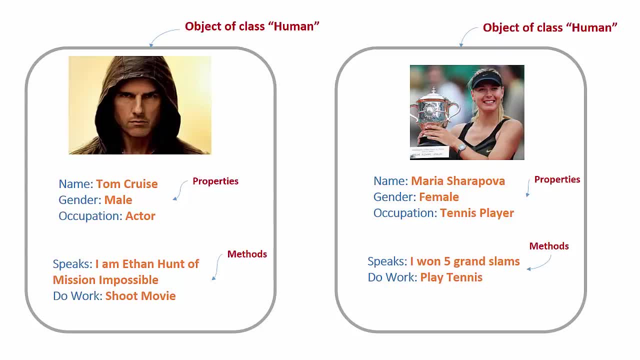 specific instance of a class, for example for human being. these two are specific instances of the human class: Tom Cruise and Maria Sarapova. they both are human beings, they both have names, gender, occupation, they both do common set of activities such as speaking, doing work, right. but when you talk about specific, 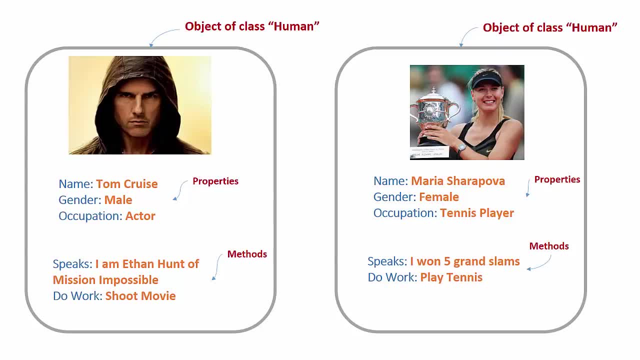 instance, the behavior, so that the behavior varies. their properties are common. for example, Tom Cruise has a name, Maya Sarapova have has a name, but when you look at the actual value, which is the real name, they are different. for example, Tom Cruise, no name is Tom Cruise and in the second case it is my. 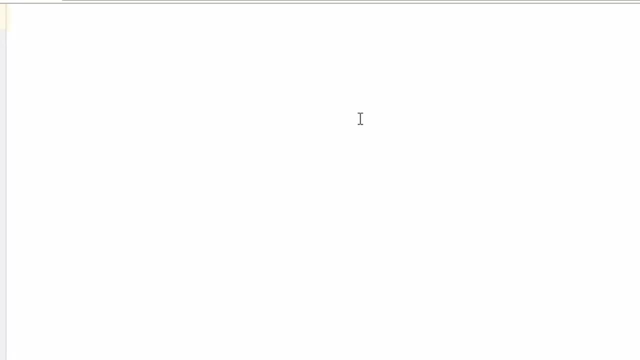 Parappa. so these names are different, but the, the properties are common. okay, as we know the concepts, now let's write our first class in Python. as usual, I have pycharm editor open and I have created class, not by file. so the way you write your class is only physical class, like this, it is ident ideological. this Ensuite I will not table. 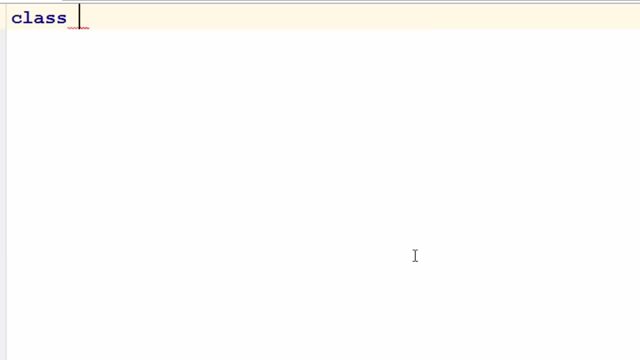 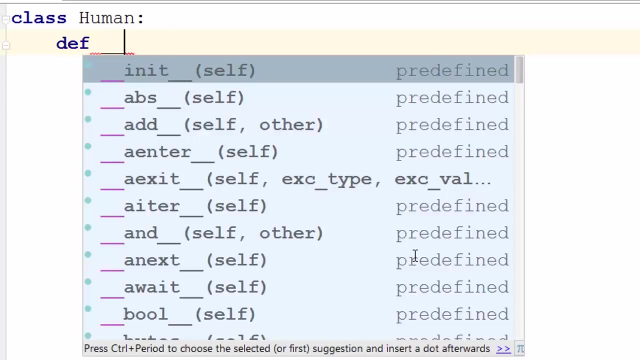 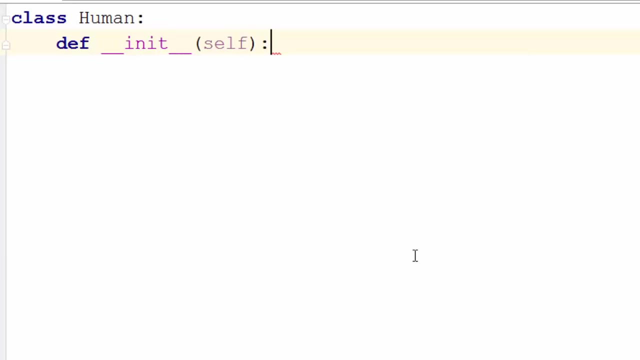 is: first, you will use a class keyword, followed by the class name, which in our case is human colon. enter the first property. the first method, not the property, is in it method. so you'll say depth, underscore, underscore in it, and it is auto typing this first argument, which is self self means, this class itself. 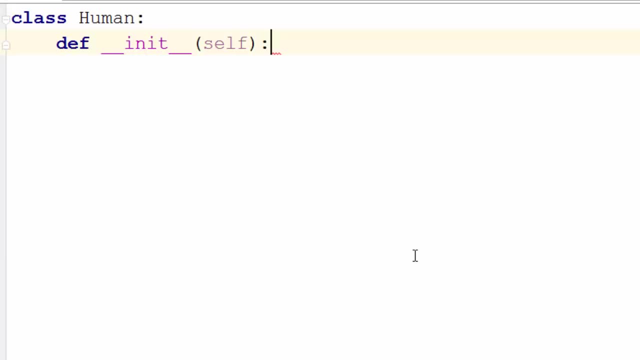 and this self is useful to define the properties of this class. and the way you define the properties, is self dot name equal to something, and you will say self dot occupation is equal to something. by doing this, I effectively define two properties in this human class, and those two properties are name and occupation. 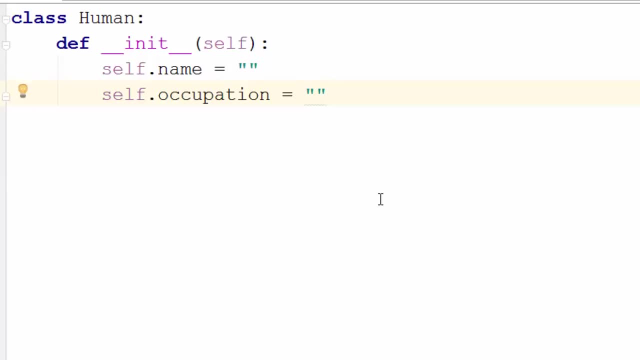 this init method will be called whenever you will create an instance of this class later on, so when you're now, as you know, from the concept that an instance has a specific value of those properties, so we need to pass those here in this function. so I'm going to pass name and occupation as an argument of this. 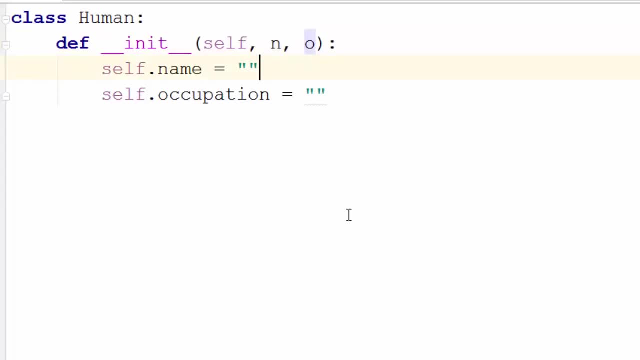 function. so I will call it n and o and assign a value of those arguments to these two properties of the class. okay, let's write our first method now, which is: do work. okay, so if you recall, from our concepts, based on the occupation of the person, that human being will be doing. 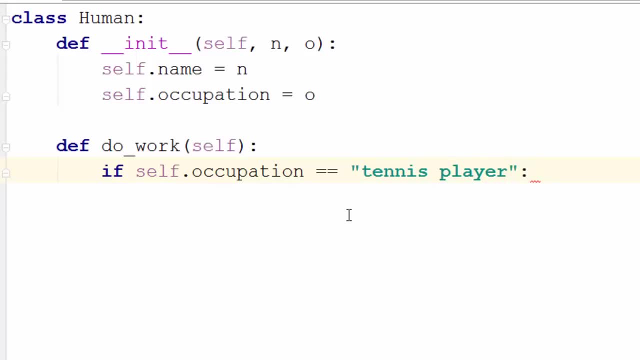 okay. so if you recall, from our concepts based on the occupation of the person, that human being will be doing different kind of work. so if the human being is a tennis player, what kind of work does he do? well, he will play tennis. right? so I will just say: plays tennis. 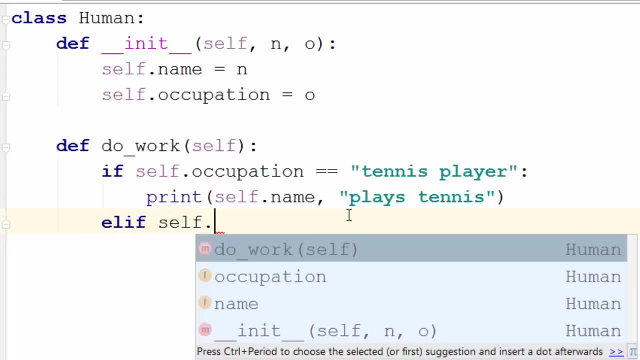 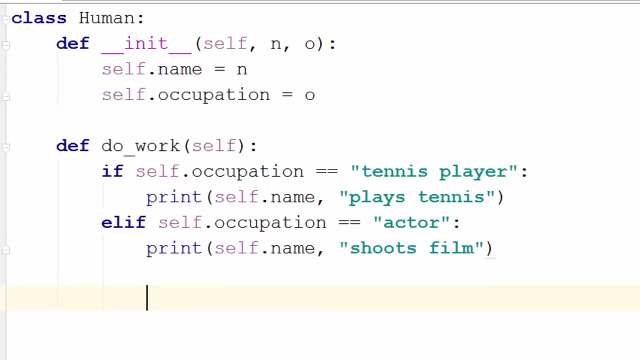 else, if the occupation of the person is an actor. what does an actor you usually do, by the way, because he cook in the kitchen. no, he shoot, it's done. usually might cook in a kitchen. okay, so this is our first master, last sight. oh, second matter, which is peaks to human being speaks. 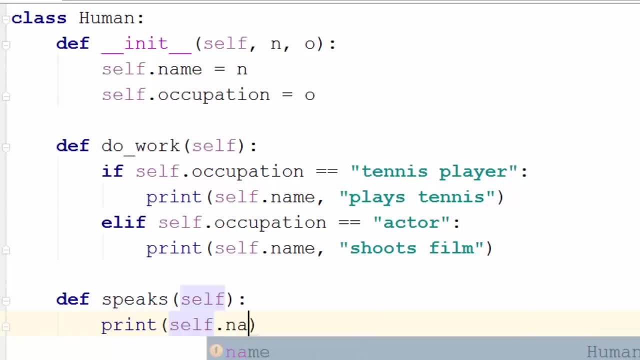 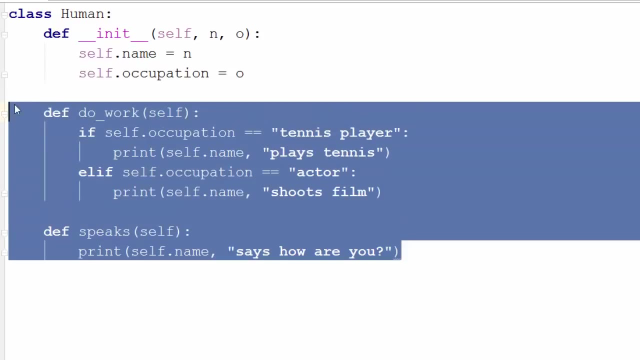 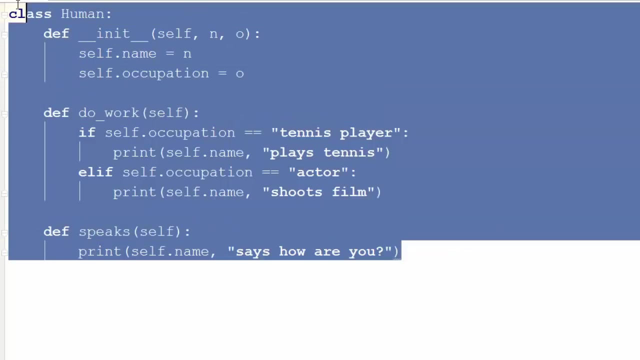 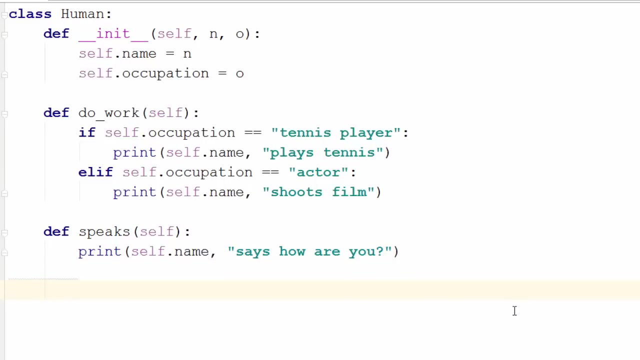 what does he speak? well, I'll say just for simplicity: how are you okay? so we effectively define two methods of the class and two properties of the class. so our class definition is complete. so this entire thing is our class definition. now let's create some instance of it. the first system I'm 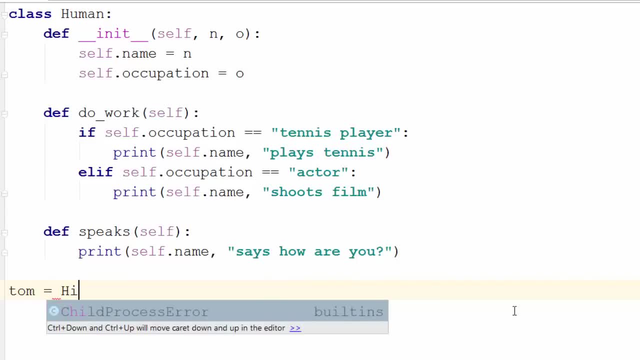 going to create is Tom, and the way you do it is you create a variable named Tom, equal to the class name, and in the bracket you will pass down those arguments. as you see in the tooltip it is saying self and O and N is highlighted, which means when you're creating an instance of a class, it is going to first. 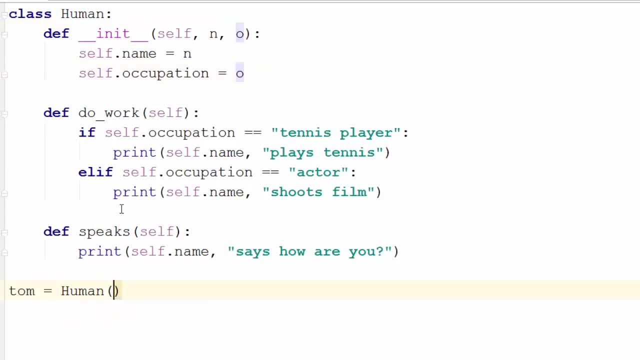 call this method init. okay, so by doing this you are calling this method, and this method takes three arguments: self, and, and. oh. but if you look into a tooltip here, it was saying that the first argument is just implicitly taken, so you need to start from the second. 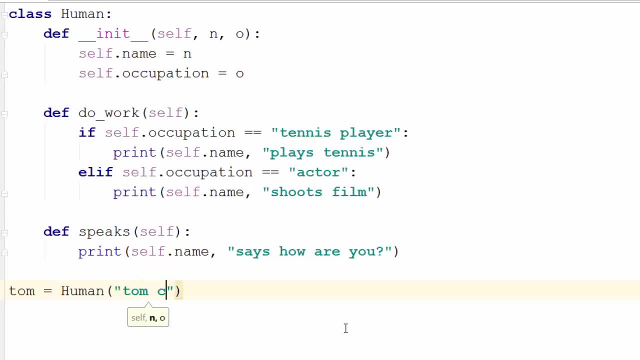 argument: okay. so in the case of Tom Cruise, it will. the name is Tom Cruise and occupation is an actor. okay, I'll say Tom Cruise and occupation is an actor. okay, I'll say Tom Cruise and occupation is an actor. okay, I'll say Tom work and Tom dot speak. okay. so I create an instance of human class and I just